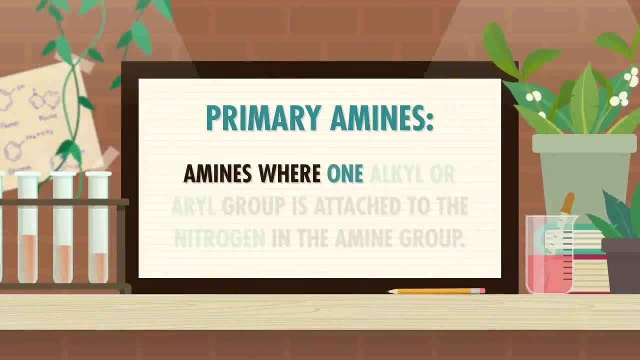 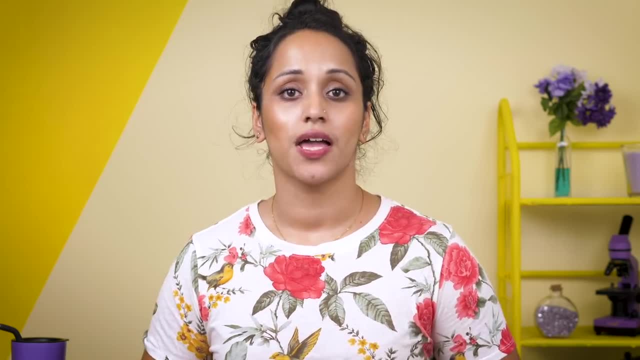 These are all examples of primary amines, Amines where one alkyl or aryl group is attached to the nitrogen in the amine group. Just like we have primary, secondary and tertiary alcohols, we can have secondary and tertiary amines too. 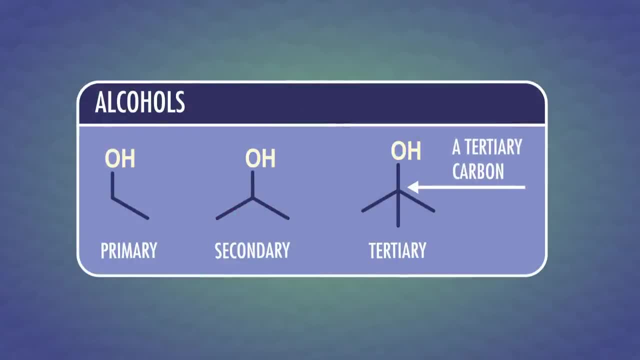 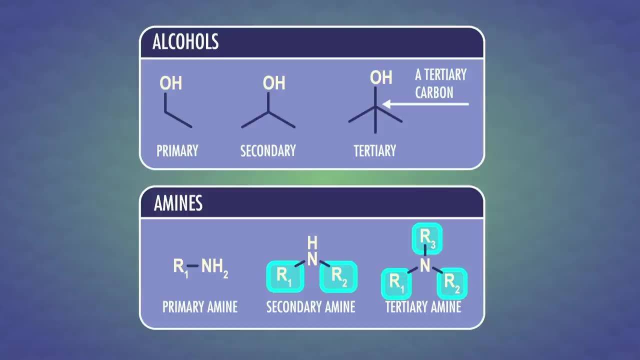 Unlike alcohols—where this refers to the carbon the hydroxyl group is attached to—a secondary amine has two alkyl or aryl groups directly attached to the nitrogen, and tertiary amines have 3 groups. Using the Common Naming System, we just list the substituent groups in alphabetical order: So a secondary amine with a methyl and an ethyl. group 2, are responsible. foraría 1, and a with alkyl are the groups that are able to remain in vanilla, although they'll often weigh a certain amount in нажung and in the amine. 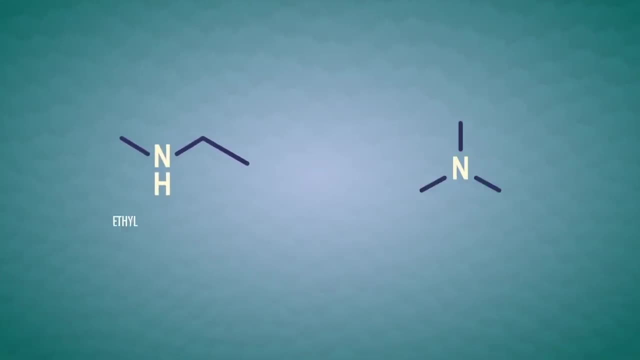 The second is when the two amines are attached to the nutrients in the same group and an ethyl group attached to the nitrogen would be ethylmethylamine, And the fishy-smelling, trimethylamine, is a tertiary amine. 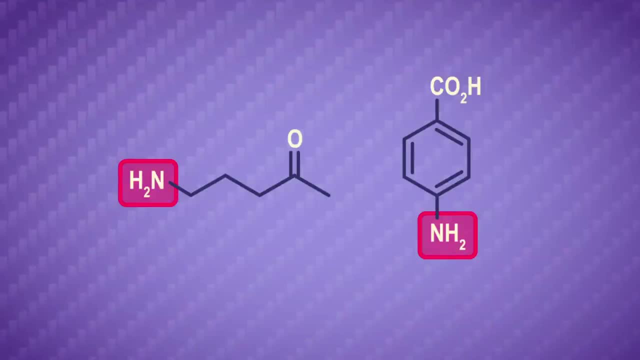 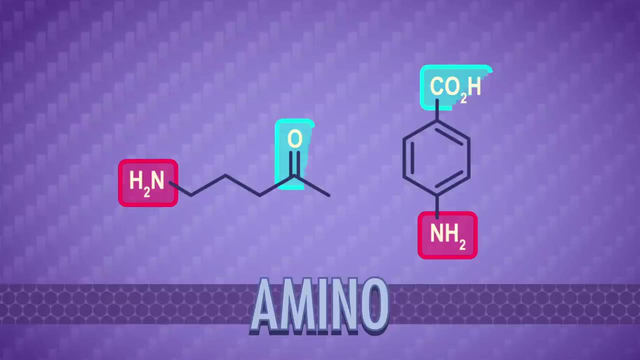 with three methyl groups attached to the nitrogen. The NH2 group is pretty low priority in IUPAC nomenclature so we'll often see its prefix name amino when there are higher-priority functional groups in a molecule like 5-amino-2-pentanone and 4-aminobenzoic acid. 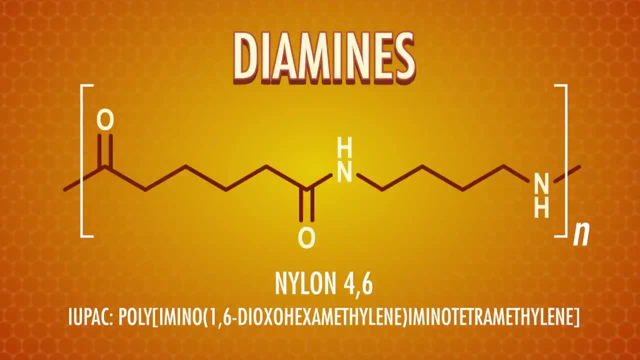 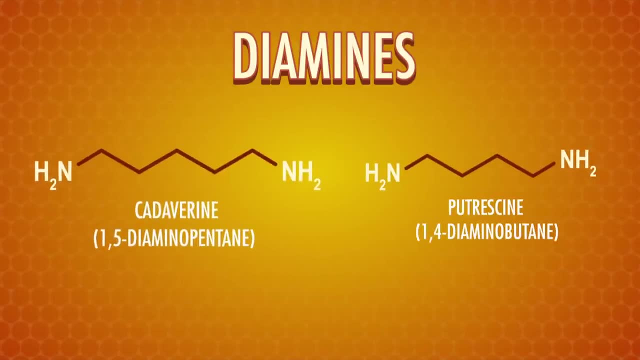 Some molecules have more than one amine group. Diamines, for example, are used as monomers to prepare some polymers like nylon from episode 31.. They're also stinky. The aptly named cadaverine and putrescine are produced when bodies decompose. 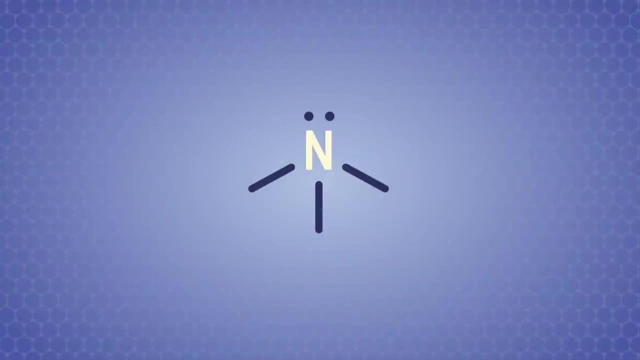 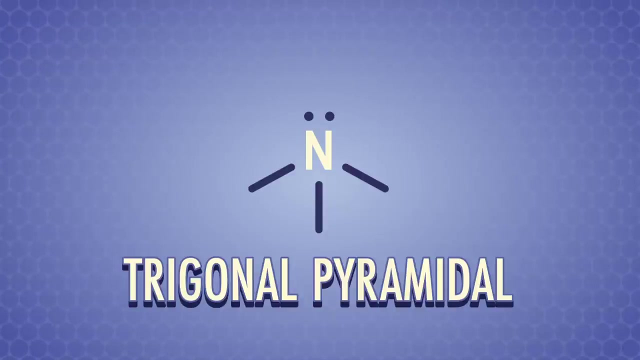 and they smell as awful as their name suggests. When it comes to shape, amine molecules have a trigonal-pyramidal geometry. The nitrogen atom is sp3-hybridized, so the electron pairs around it. take up a tetrahedral arrangement, like we see for carbon. 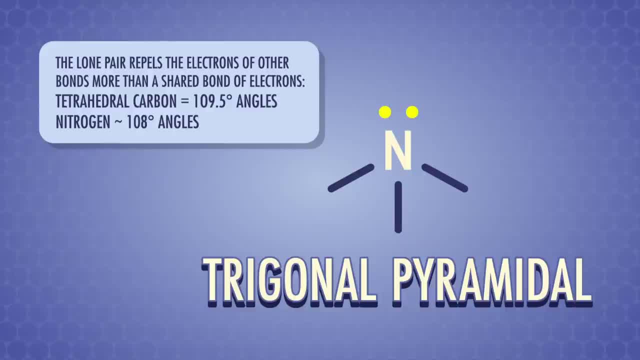 Unlike carbon, though, nitrogen has a lone pair of electrons, taking up a tetrahedral arrangement like we see for carbon. They take up the fourth spot, giving the atoms the pyramidal shape, And in chemical reactions, amines are weak bases. 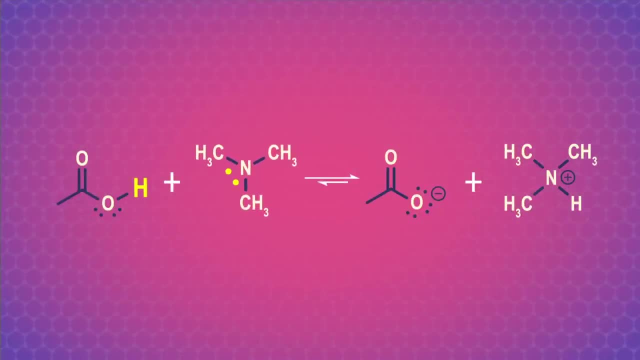 The lone pair of electrons on the nitrogen can accept a proton, forming the conjugate acid, an ammonium ion. Looking at the pKa of the ammonium ion we generate tells us how basic the amine is. Remember, a low pKa means a compound is more acidic and more willing to give up a proton. 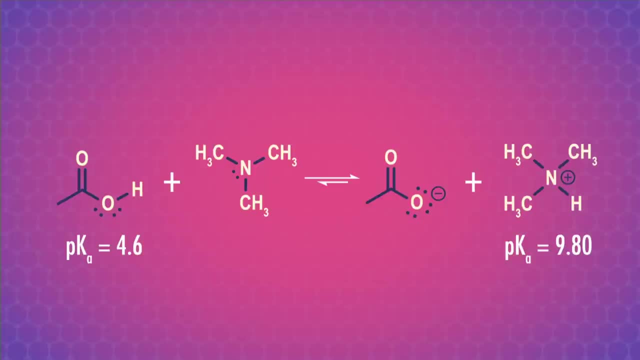 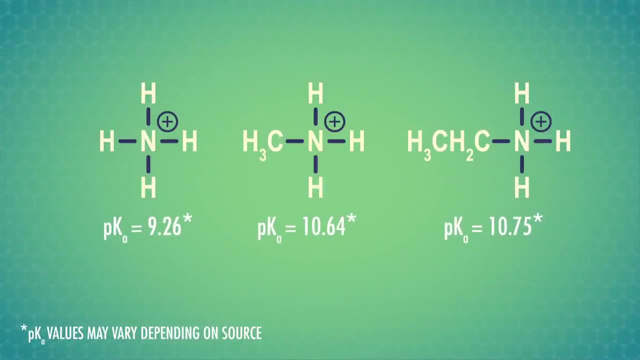 So if an ammonium ion has a higher pKa, this means the original amine is more basic and more willing to accept a proton. If we want to increase the basicity of an amine, we can substitute in additional alkyl groups. 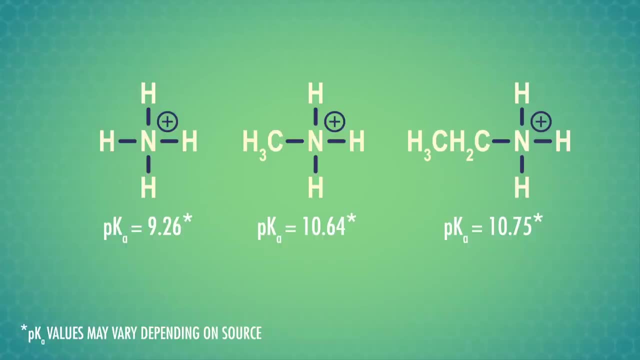 Remember that alkyl groups are electron-donating, So when an amine picks up a proton to become a positively charged ammonium ion, the alkyl groups help stabilize the positive charge. We can see this effect in action when we compare the pKa values. 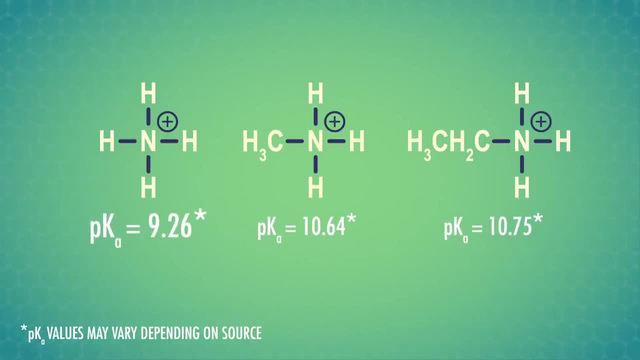 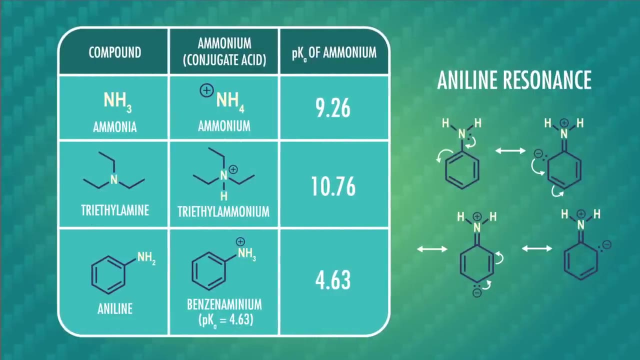 of alkyl-substituted ammonium ions to the simple ammonium ion. The basicity of amines can also be affected by resonance. For example, aniline, which is an amino acid, can also be affected by resonance, And acetylene, which is a precursor of the indigo dye used in blue jeans. 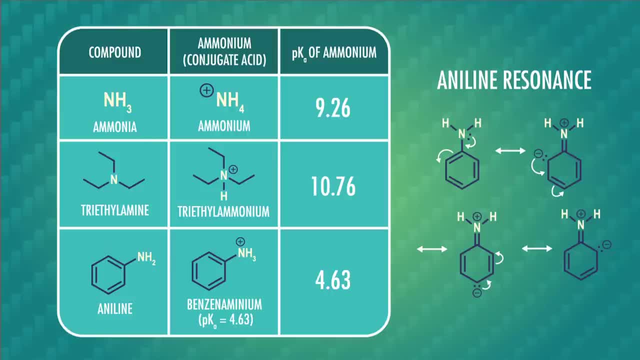 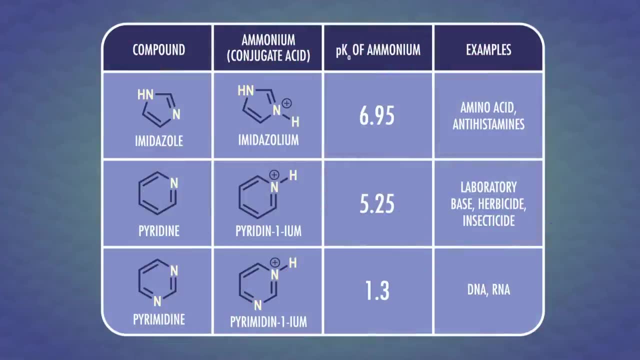 is a much weaker base than alkyl amines. This is because the nitrogen lone pair is tied up in the resonance in the ring. There are also nitrogen-containing heterocycles, which are cyclic molecules with nitrogen and at least one other element in the ring. 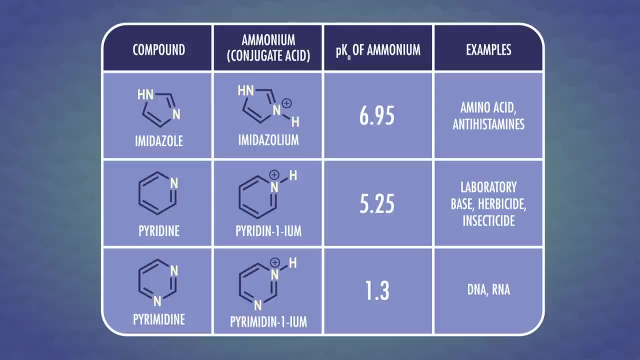 When the cyclic compound isn't aromatic. these amines have basicities comparable to alkyl amines. However, nitrogen-containing aromatic heterocycles are much weaker bases than alkyl amines because of sp2 hybridization of the nitrogen. 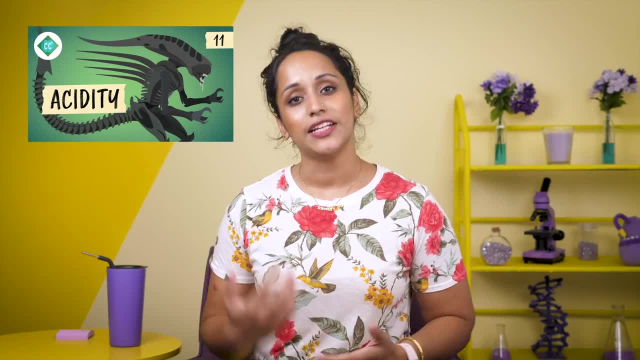 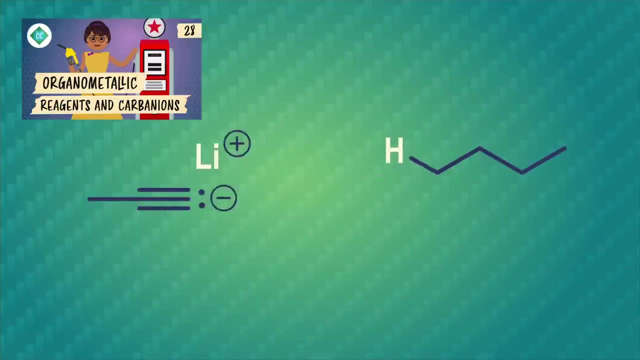 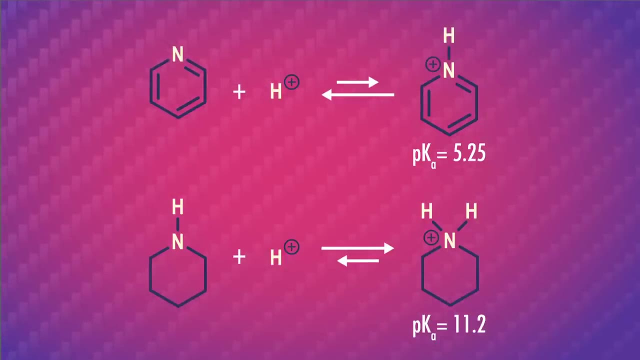 We saw how increasing S-character increases the acidity of the hydrogen on a carbon. That's why we can deprotonate the hydrogen atom on a terminal alkyne. But in this episode we're looking at amines, And protonated sp2 nitrogens lose their protons more easily than protonated sp3 nitrogens. 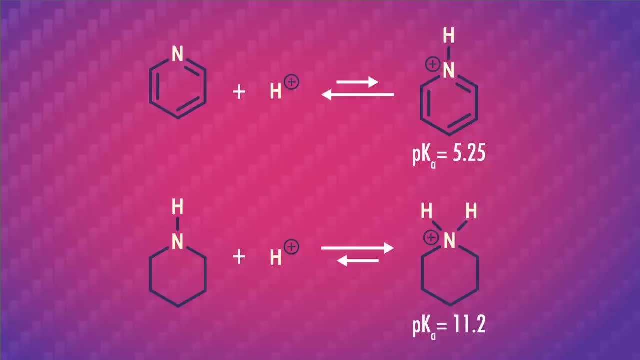 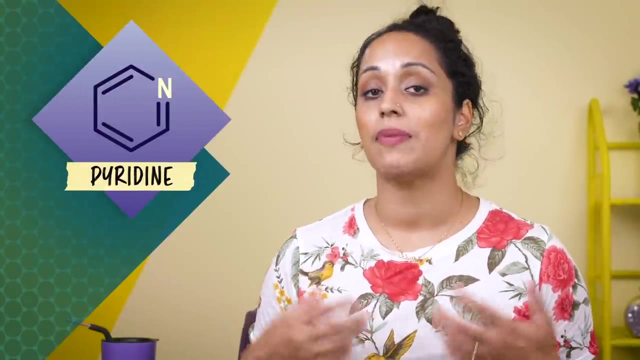 So sp2 hybridization makes the conjugate base, the unprotonated amine, less basic. One of these heterocycles, pyridine, is a super useful molecule in the lab as a precursor. It's used to produce herbicides such as paraquat, as well as insecticides and antiseptics. 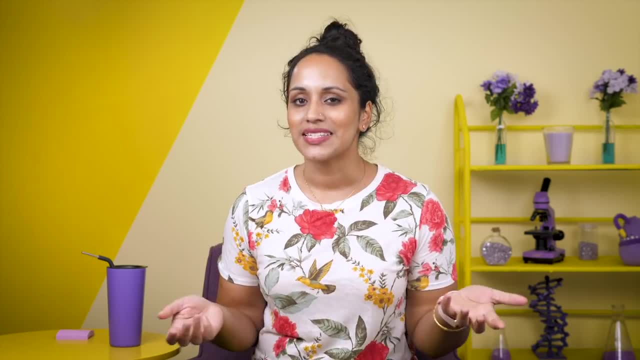 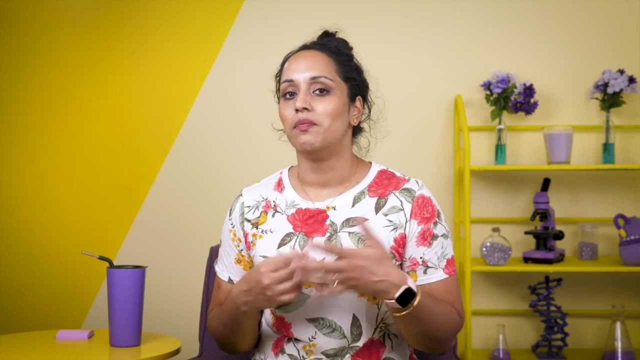 If you need to use it, though you might want to hold your nose, Sensing a pattern here. Pyridine's aroma has been diplomatically described as very characteristic and, more bluntly, as sour and putrid. So now that we really know what amines are and what they can do, 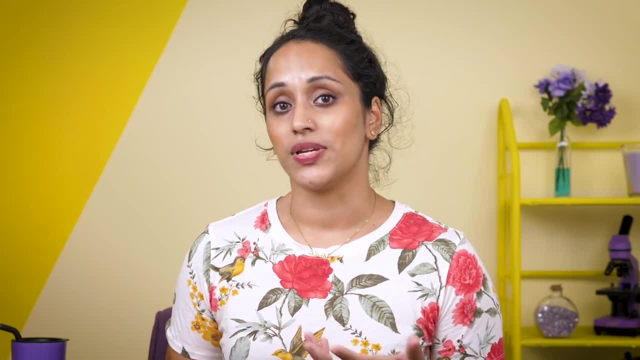 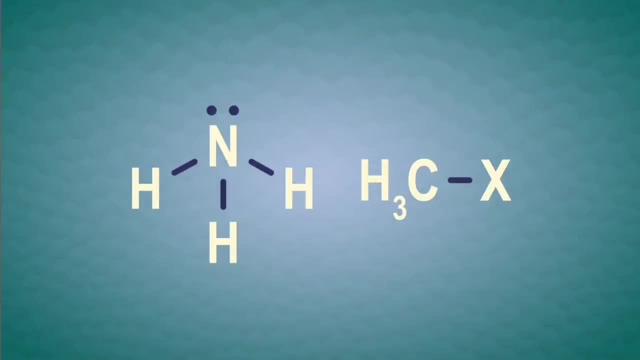 let's talk about how we make them. There are a few ways we can do this using a combination of nucleophilic substitution reactions and reductions To make an amine. the simplest nucleophilic substitution is reacting ammonia with a haloalkane. 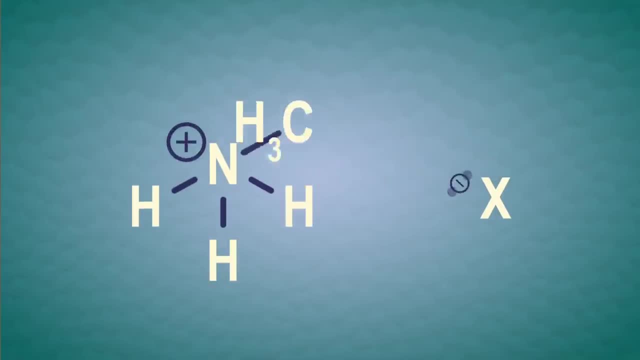 The lone pair on the nitrogen grabs the alkyl group from the alkyl halide to make an ammonium ion And by adding a base to remove the extra proton we get a primary amine. But there's a little problem with this reaction. 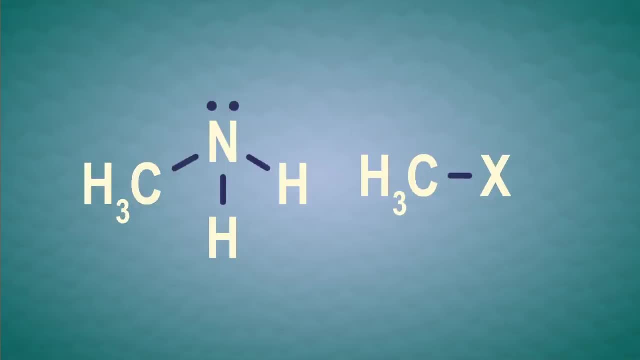 It just keeps going. Remember that more substituted amines are more basic than ammonia, which also makes them more nucleophilic. So the primary amine grabs the alkyl group from the alkyl halide to make an amine, And so on. 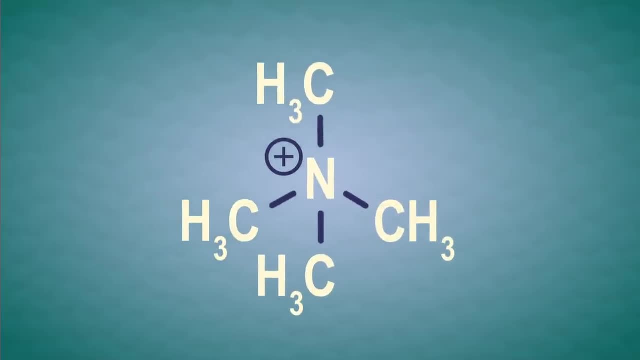 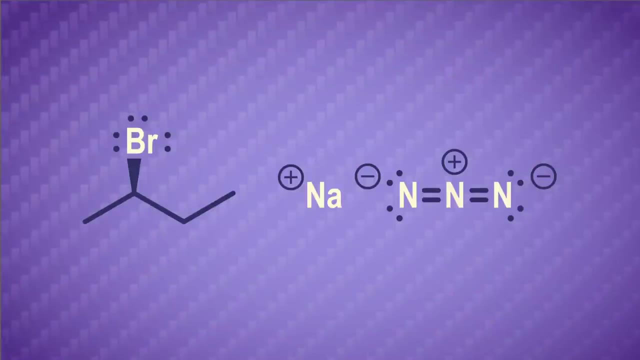 We end up with a quaternary ammonium ion, a positively charged nitrogen surrounded by four alkyl groups. Not great, if we just wanted a primary amine. This over-alkylation problem can be solved by converting the alkyl halide to an alkyl azide. 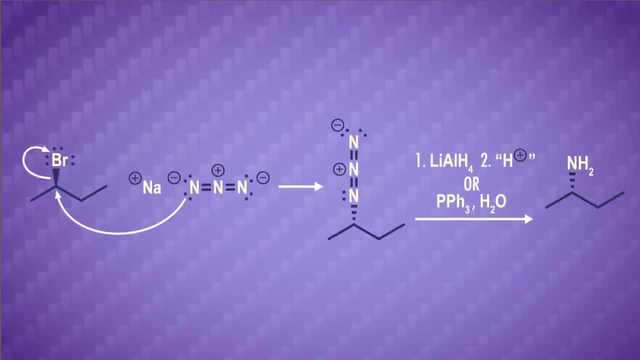 another nucleophilic substitution reaction. We can then reduce the alkyl azide to produce an amine. But there's an issue with this reaction too. The alkyl halide is a nucleophilic substitution reaction. So the alkyl halide is a nucleophilic substitution reaction. 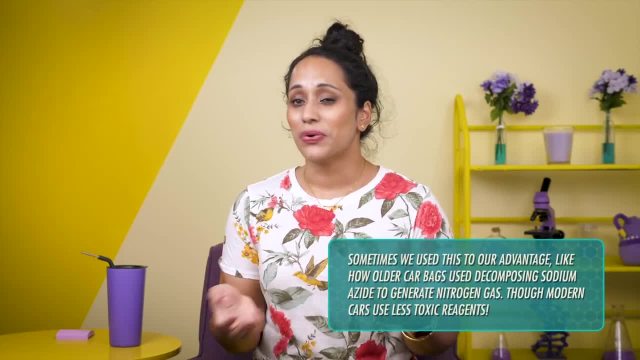 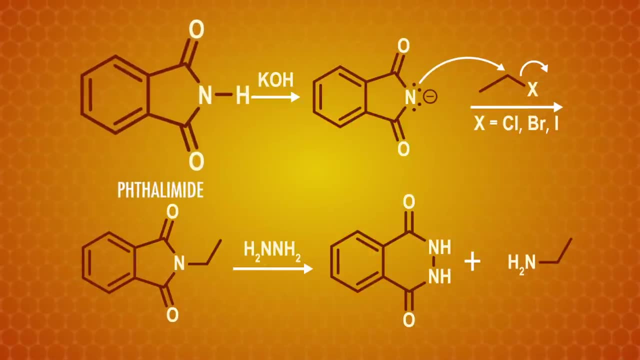 Besides, particularly ones with low molecular weights can be explosive if they're not in solution. A third method is named the Gabriel synthesis after its discoverer. This uses the compound thalamide to add nitrogen, And it's pretty cool because it adds a built-in amine protecting group at the same time. 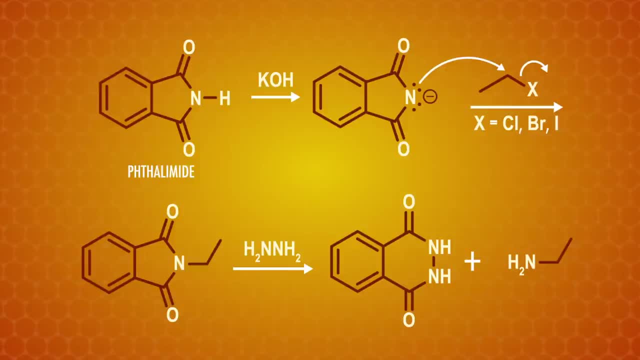 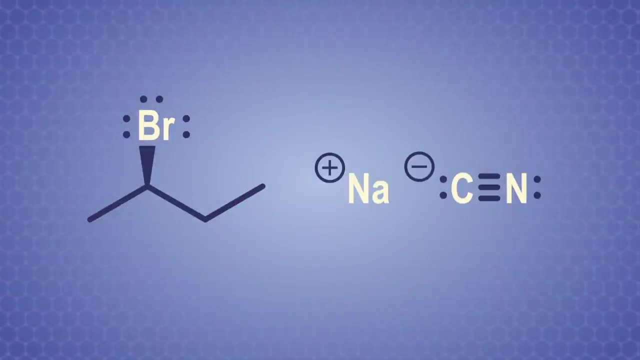 We actually saw this protecting group in our penicillin synthesis in episode 33.. To remove that and get our primary amine, we can react the compound with hydrazine. A fourth option to get a plain old primary amine is reducing a nitrile. 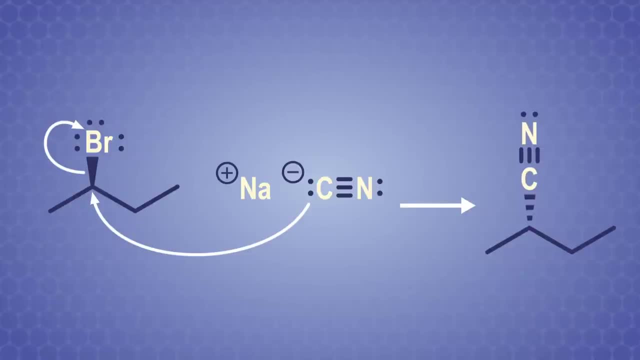 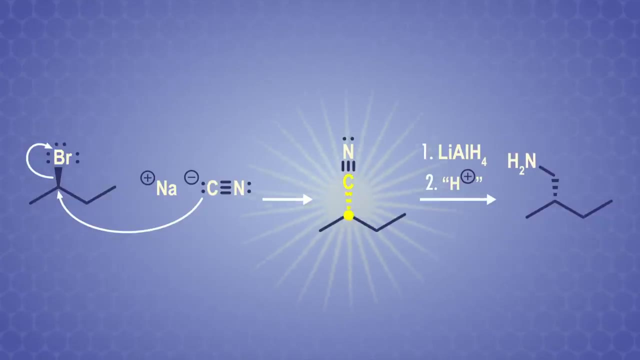 Like the azide reaction. the first step is nucleophilic substitution with the haloalkane. Then we can reduce the nitrile group to a primary amine. We also get a bonus carbon atom with this strategy. And lastly- in episode 32, we learn that we can make amines. 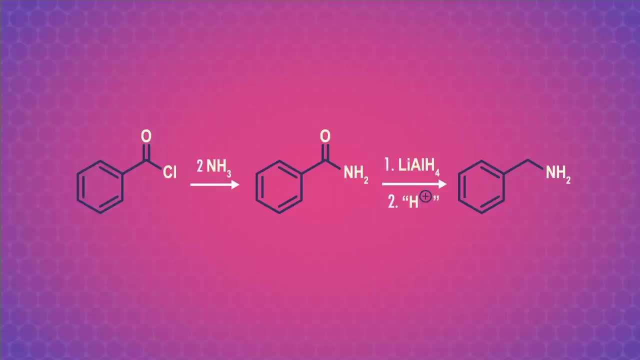 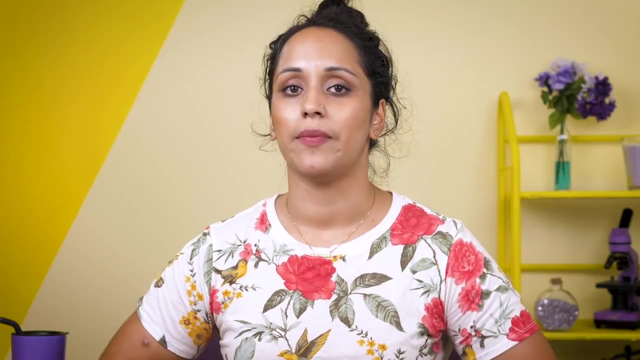 by reducing amides with lithium, aluminum hydride. As a reminder, we can make the amides easily from acid chlorides or esters. Up until now, we've only made primary amines, But amide reduction also gives us a path to secondary amines. 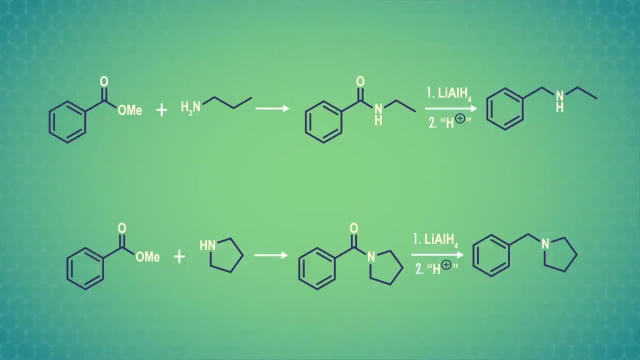 We just need to make an amide with alkyl groups substituting in for the hydrogen atoms. Reacting an ester with a primary or secondary amine allows us to do just that, And reduction gives us the secondary or tertiary amine we're after. 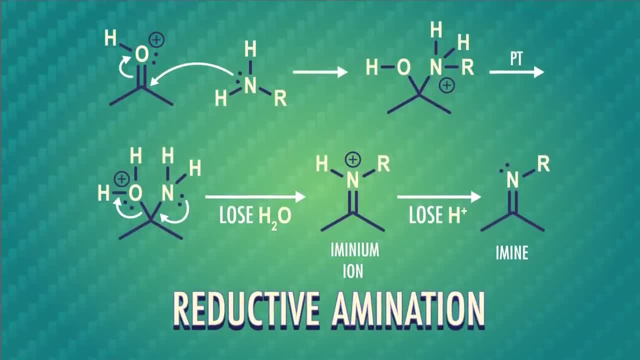 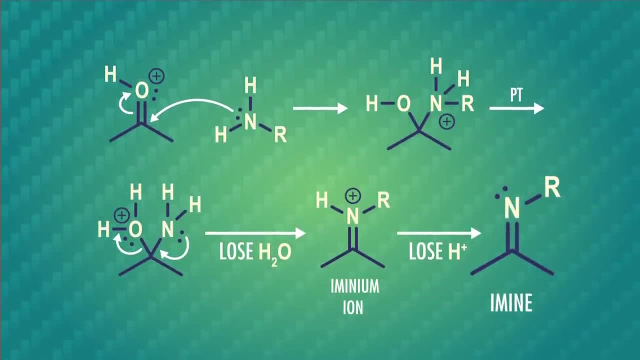 There's also a reaction called reductive amination, which uses a milder reducing agent to add additional alkyl groups to an amine. Remember imines. They're molecules with a carbon-nitrogen double bond made by reacting ammonia or a primary amine. 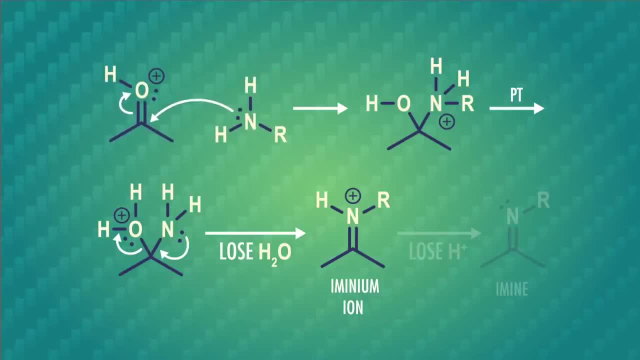 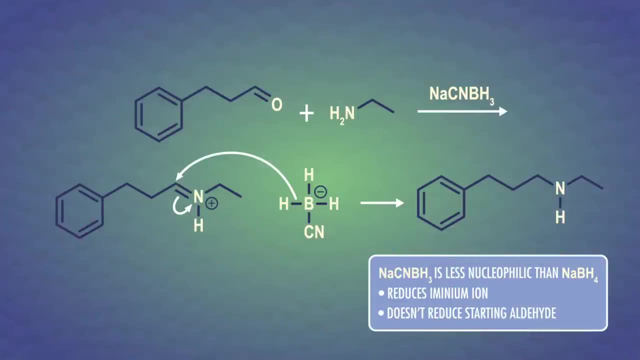 When making imines, nitrogen swaps out for the oxygen of an aldehyde or ketone, and we first get an iminium ion. In reductive amination we then add a hydride to the electrophilic carbon of the iminium ion. 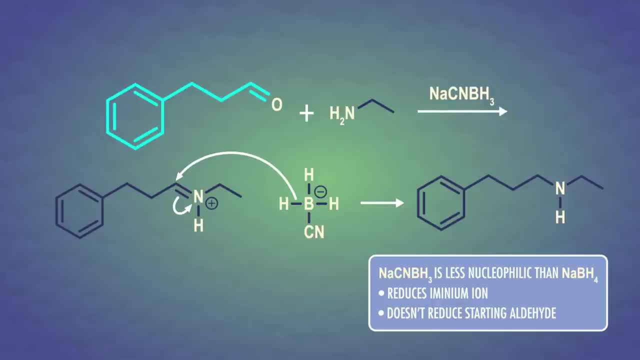 with a mild reducing agent. The alkyl group, originally attached to the carbonyl group, is now attached to the nitrogen. This is where we can customize what gets added to the amine simply by changing the alkyl group attached to the carbonyl compound. 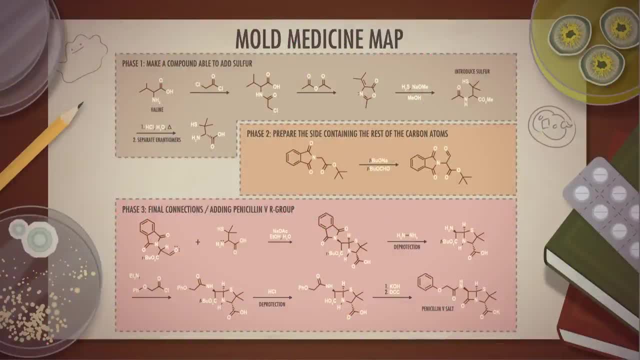 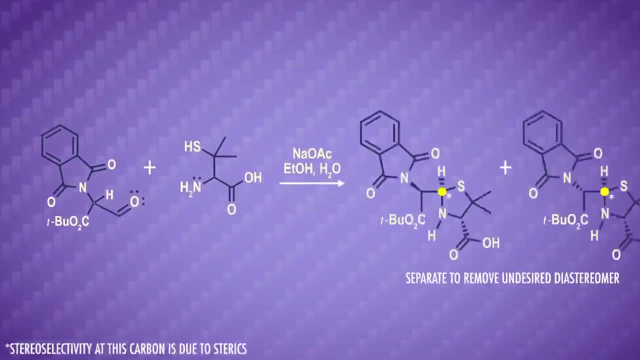 While we're talking about iminium, we should highlight where they play a role in our mold medicine map of penicillin V. This step uses a similar reaction to close one of the rings, Like the reductive amination reaction we just saw. 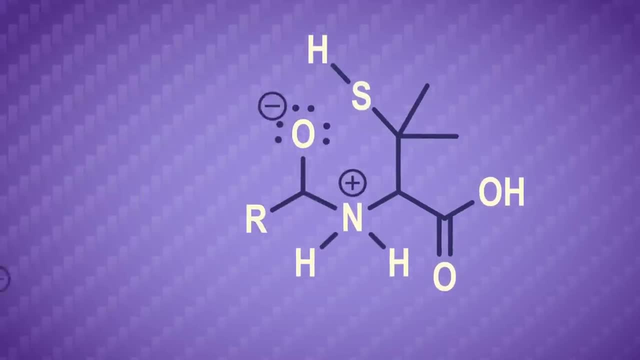 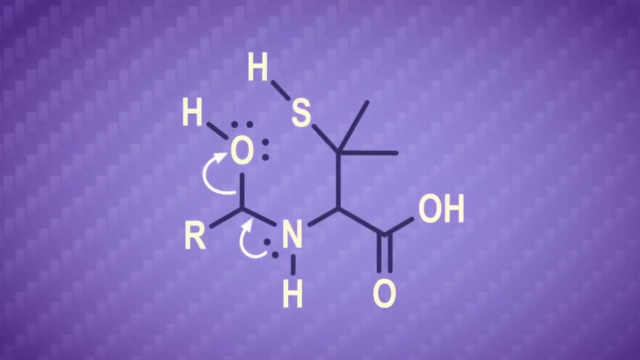 the lone pair on the nitrogen attacks. the carbonyl carbon A proton jumps to an acetate ion which is grabbed by the negatively charged oxygen. Then we lose the hydroxide ion to form the iminium ion. So far, so good. 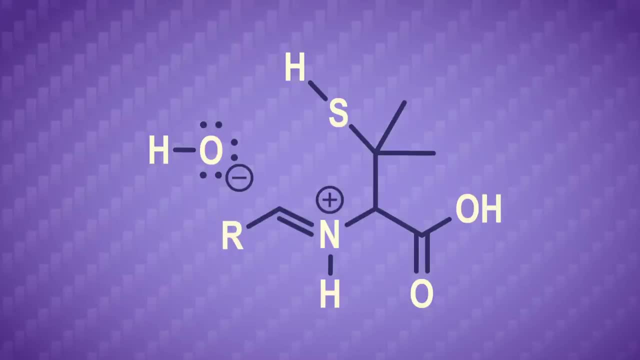 Now lots of different nucleophiles can add to iminium ions, not just hydride, like we saw before Here. the hydroxide ion we just kicked out can grab the hydrogen from the thiol group and the sulfur attaches to the iminium ion carbon. 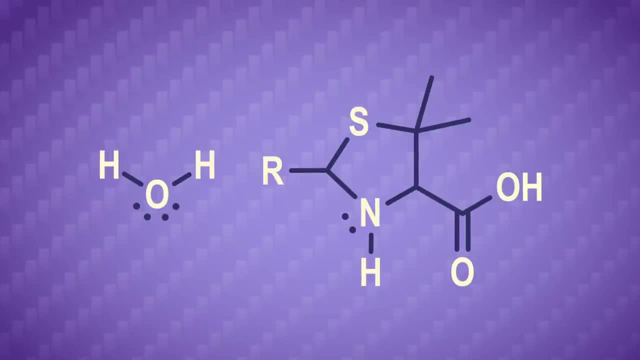 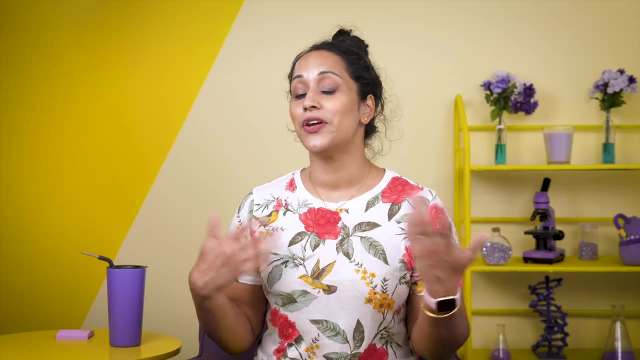 And there you have it. We've closed the five-membered ring in penicillin V. Filling in more of our mold medicine map is cool and all. but we have a couple more amine-forming reactions to explore. I know I said that over-alkylation can be a problem sometimes. 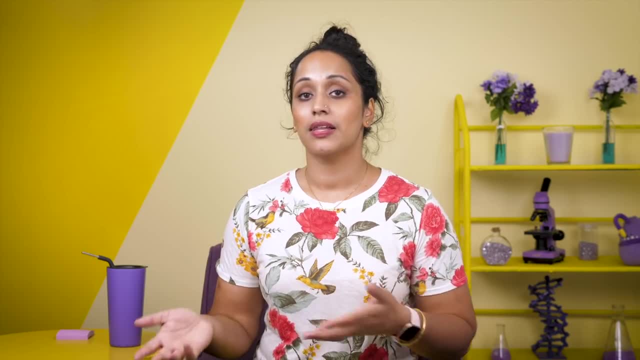 but an over-alkylated amine can be useful too, Like quaternary ammonium salts are pretty good, leaving groups. If we take a quaternary ammonium salt, we can get a quaternary ammonium salt. 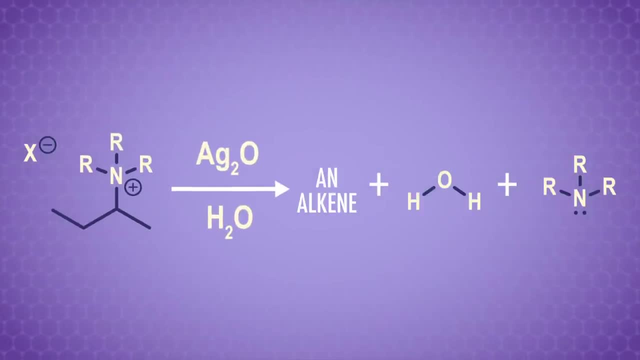 which is a pretty good leaving group, If we take a quaternary ammonium salt. we can get a quaternary ammonium salt, which is a pretty good leaving group, If we take a quaternary ammonium halide and heat it with silver oxide and water. 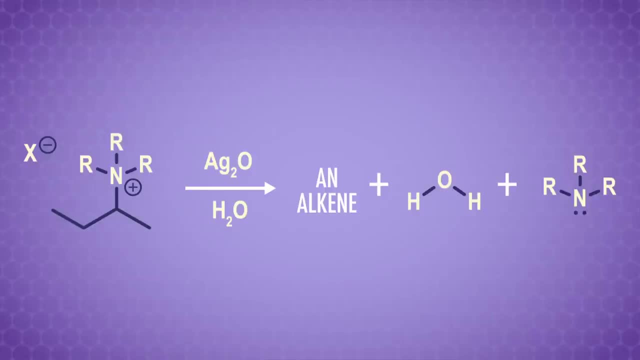 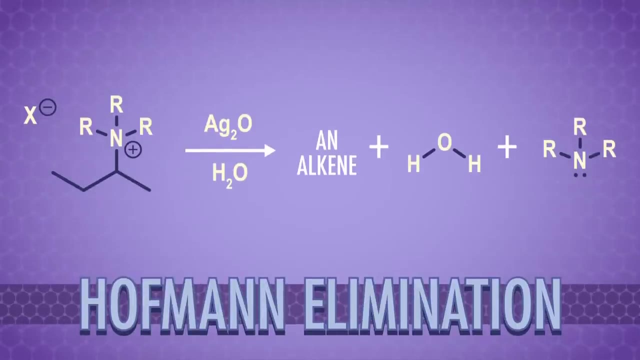 a hydroxide ion plucks off a proton as the nitrogen leaves, giving us an alkene water and a tertiary amine. This is known as the Hoffman elimination, named after the chemist who discovered the reaction. Hoffman elimination is unusual because the major alkene it produces 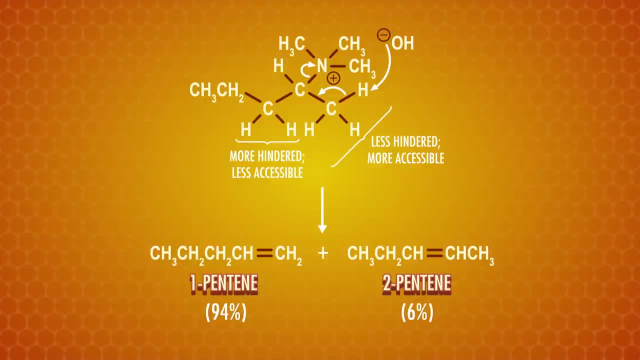 is the least stable alkene possible. Most other elimination reactions favor the more stable alkene. This quirk is because of the bulky tertiary amine leaving group. It sterically hinders the reaction, but it's not always the case. It also hinders the transition state for the more stable alkene. 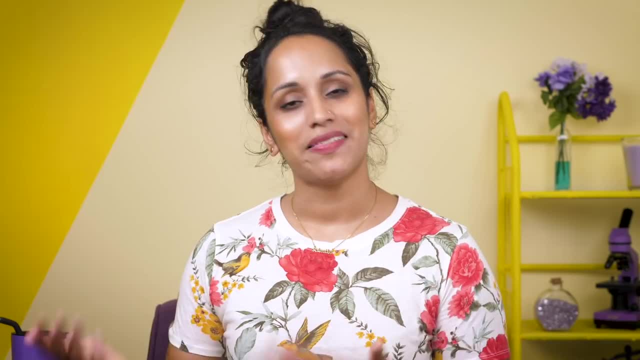 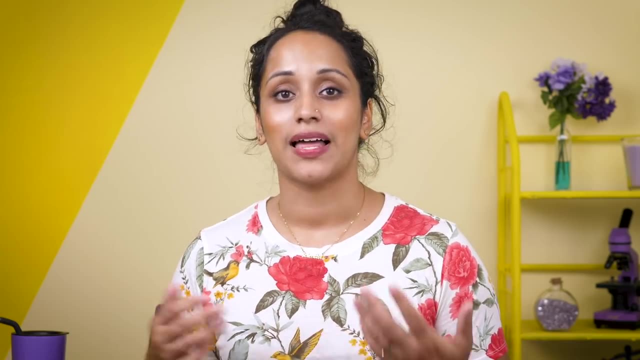 and therefore paves the way for the alkene that's less stable. And then there are enamines, which contain a carbon-carbon double bond next to an amine. Remember, they're an alkene plus an amine. Back in episode 29, we talked about forming enamines. 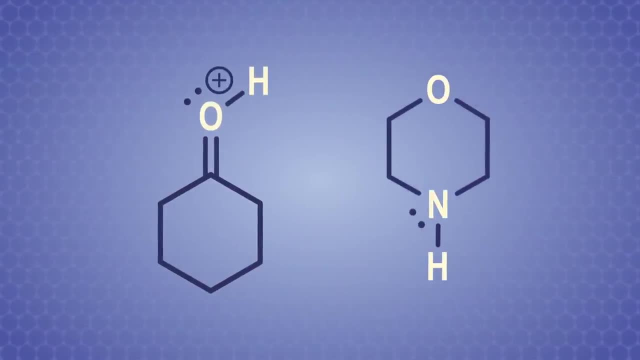 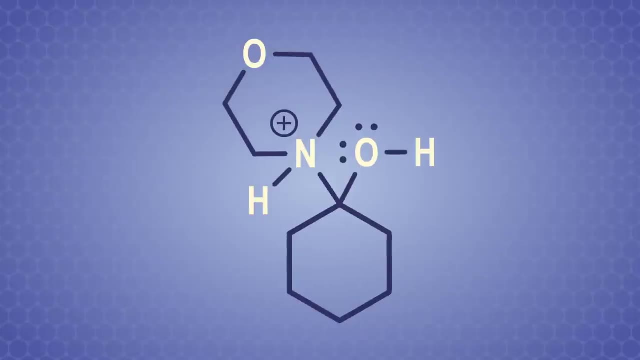 by reacting an aldehyde or ketone with a secondary amine which, as we mentioned earlier, has two alkyl groups attached to the nitrogen. The first few parts of this reaction are identical to the imine-forming reaction that we've done a couple of times. 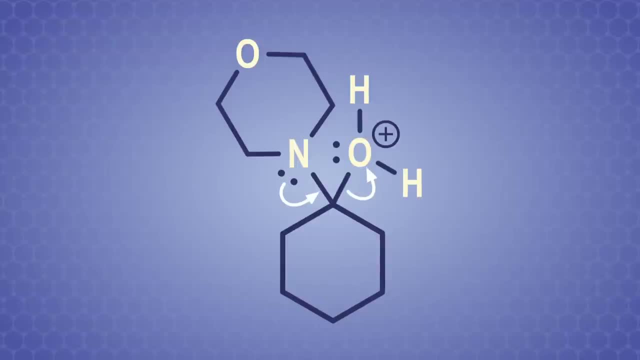 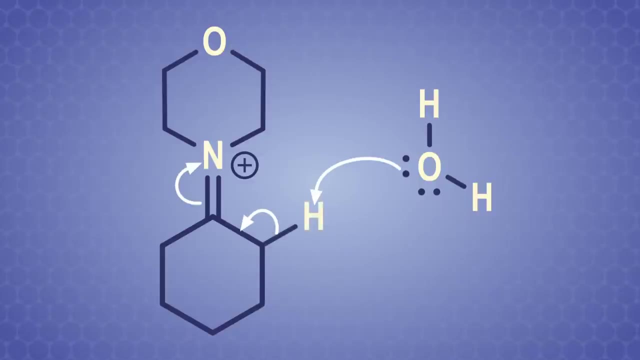 already in this episode. However, after water is eliminated, the secondary amine doesn't have an additional proton to lose to form an imine. So a proton is lost from the carbon adjacent to the one attached to the nitrogen. instead, Now we have the enamine. 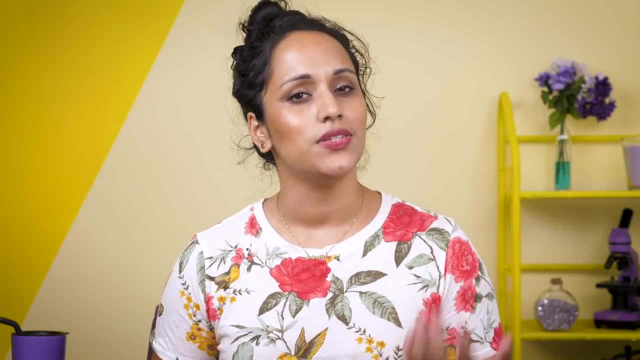 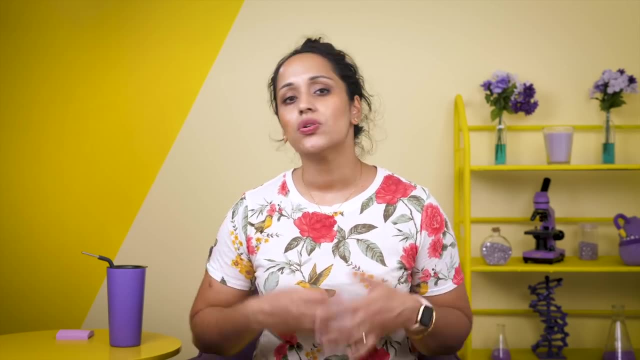 Now what we didn't talk about in episode 29 is what we do once we have an enamine. Turns out they act as nucleophiles in the same way as enolates and give us carbon-carbon bonds, So we can use them in the same kinds of reactions like alkylation. 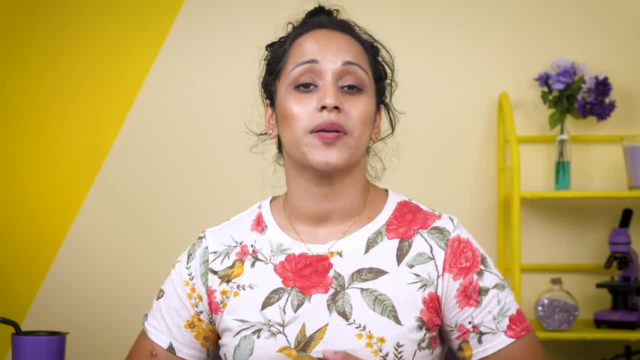 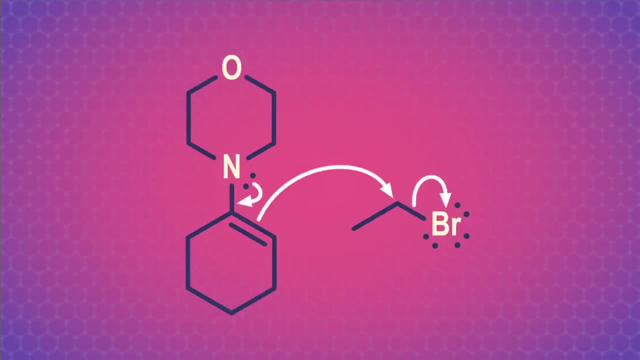 They have some advantages over enolates because we usually don't have to worry about over-alkylation. Take a look at this mechanism. The nitrogen-lone pair pushes down to help the double bond attack the halide in a nucleophilic substitution reaction. 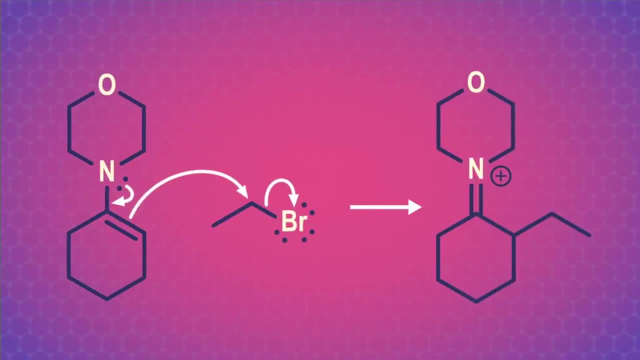 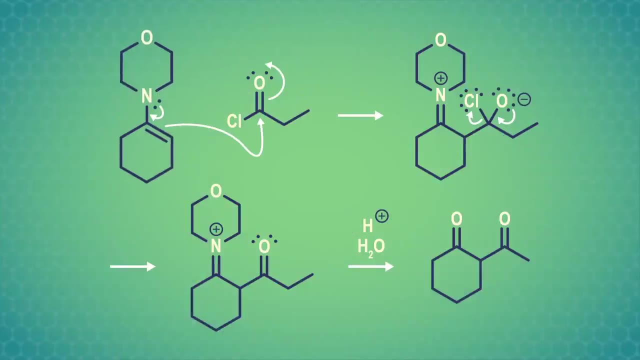 We get an iminium ion as an intermediate which can't react more than once, So we can easily stop the reaction here, Not like the enolates we made in episode 43. We can use enamines for acylation reactions. 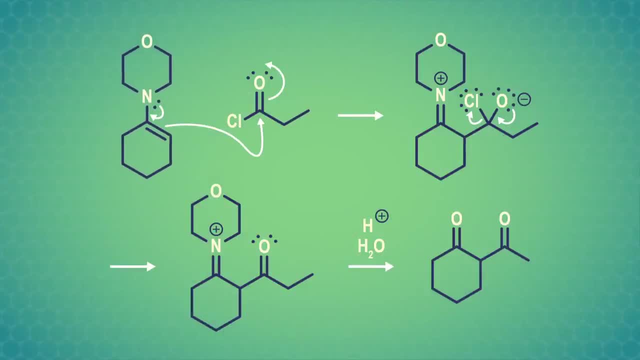 which enolates do too, In both alkylation and acylation reactions with enamines. we reform an iminium ion through the course of the reaction, which we then hydrolyze in the final step to reform an aldehyde or ketone.